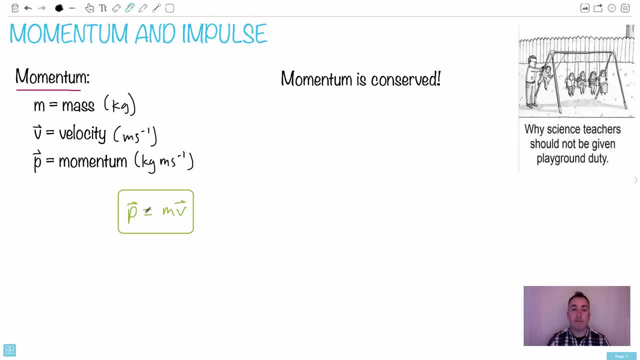 goes missing and gets turned into energy and weird stuff. there. Velocity isn't necessarily conserved from before to after. Somebody figured out that if you multiply mass and velocity, just that product of mass and velocity, that thing we call momentum, that thing that's. 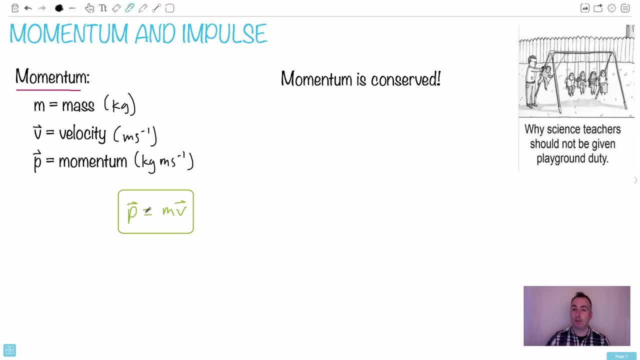 kind of arbitrary that is conserved. so that's what we use. this is a reason why it's a useful unit. okay, because momentum itself by it, on its own, doesn't really mean much to us. it's a product of mass and velocity, yes, so what? well, the reason. 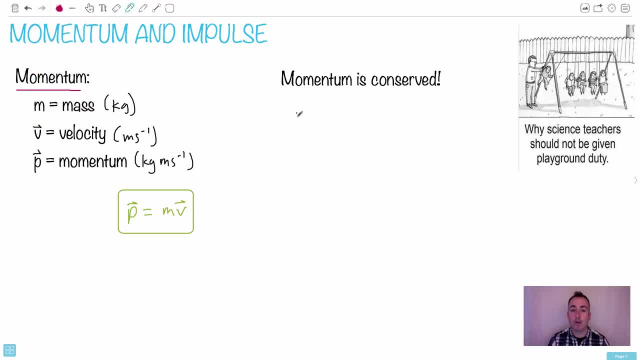 why it's important is because of this idea here that it's conserved, which means the momentum before, like the total momentum before, will equal the total momentum after, and you use this to make predictions. you can use this to solve all sorts of crazy problems. so this is the main idea behind momentum. 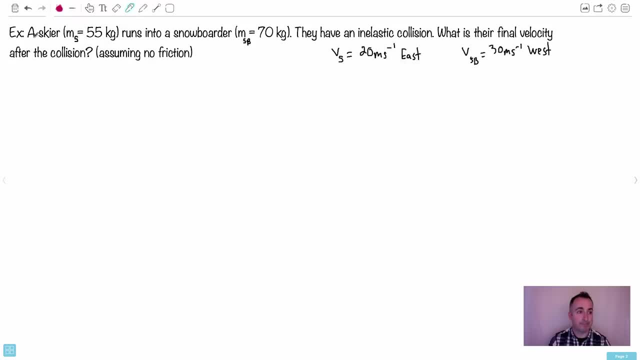 conservation. so I'm gonna give you an example here. I just went skiing recently, so that's why I was thinking about this. but I mean it's very much set up like an IB question. I just changed the skier and snowboarder, but I mean the idea is an. 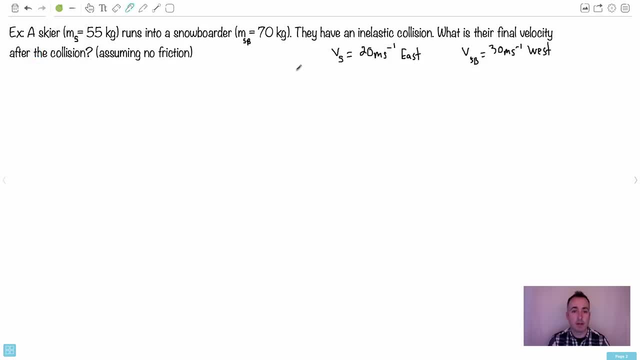 IP idea here. they definitely do this. so let's just split everything. I like to split the question into two here. so we have a skier. mass of the skier is 55 kilograms and they run into a snowboarder of 70 kilograms. they have. 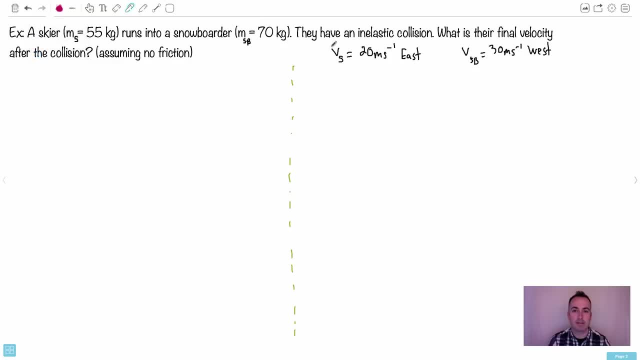 an inelastic collision. do you know what inelastic means? inelastic means they don't bounce. in other words, they stick together. they stick together. that's the important thing here. inelastic means they stick together. now what's their final velocity after the collision? assuming no friction, and we're given. 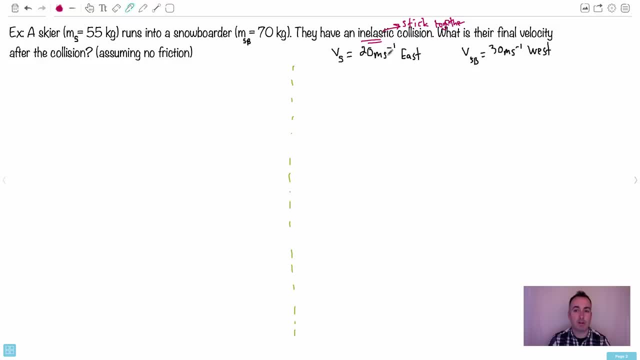 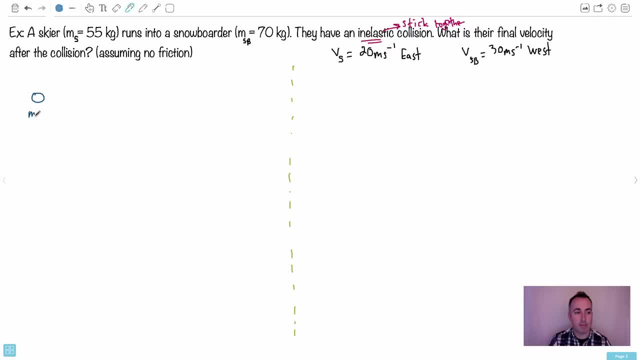 artist. I'm just gonna say this: is it gonna be the skier and it's gonna be M? skier is 55 kilograms and I have V. skier is what was it? again, it was 20, so 20 meters per second, and I'll draw East, being that way, just to the right now. I'm 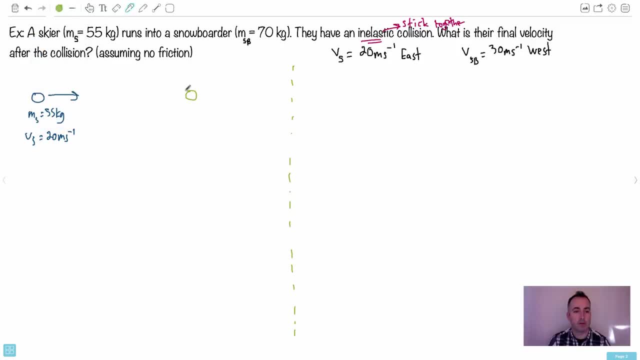 gonna draw the snowboarder. this is a snowboarder over here. they're going to left. by the way, I'm gonna set a mass of the snowboarder is 70 kilograms. I'm just lining everything up, just it's gonna be a lot easier to deal with and the 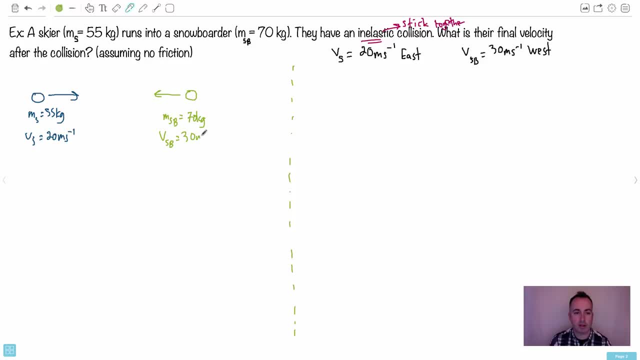 velocity of the snowboarder is 30 meters per second. now, what's really important, then, is: I met me again, if you want to figure out what happens. I mean, in the end, here they stick together of this person and we have the skier here, right? 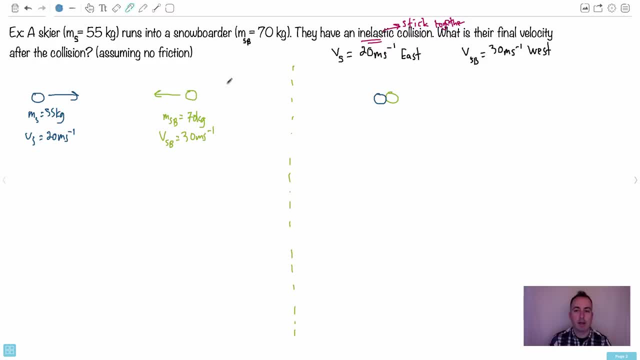 they're stuck together somehow, so maybe they're sort of tangled and they're angry with each other. now we don't know what, necessarily which direction they're gonna be going. we're going to figure that out, but we want to know their final velocity, and a good way to do that is again to calculate. what is the thing. 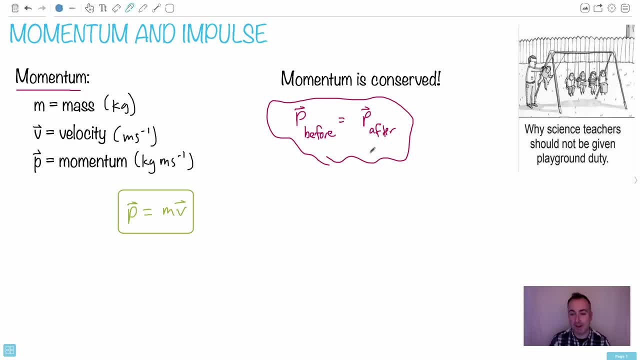 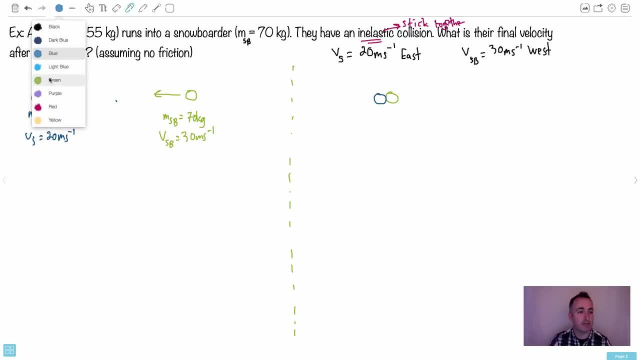 that's conserved and obviously you should know it, since it's a video about momentum. duh, he's probably gonna use a momentum example, but this is an example where we need momentum, so let's actually find it here. so I'll try to solve for a. 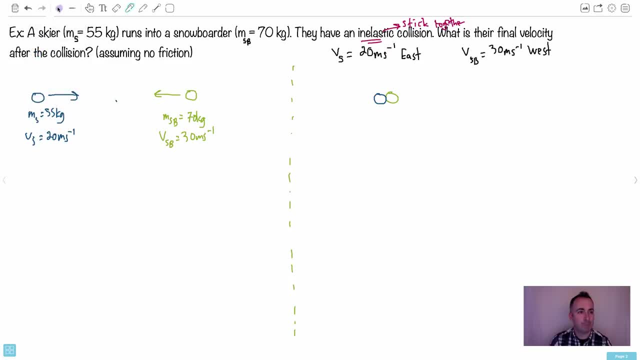 momentum. here I'll say I don't want the same colors, maybe, so I have momentum of the skier. well, the momentum is just mass times velocity, so it's just 55 times 20, so that's a hundred, no hundred, 10, with the extra zero there: kilogram meters per. 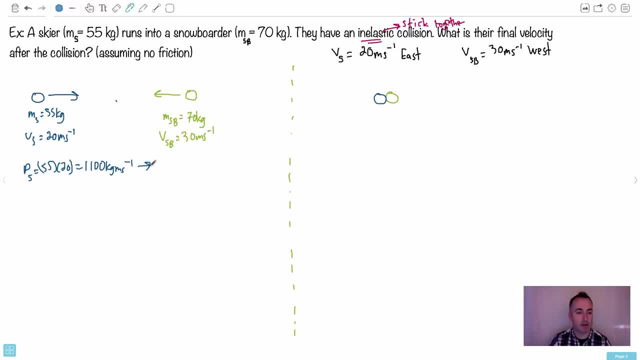 second, and that is in the direction of the travel. so that's Boe. now we also have the P of the snowboard, the momentum of the snow border. let's figure that out. that is 70 times 30, which is 21 with two extra zeros. so this is this number here, right, yeah, kilogram meters per second, that's. 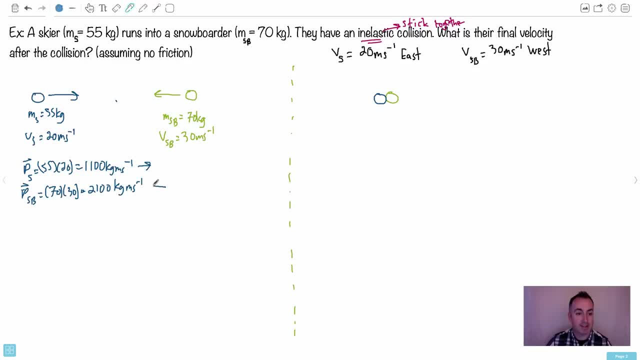 the momentum of the snowboard percent. but this is that way it's left. now it helps to figure out what's the total momentum. then. total momentum, lcp, total- it's just going to be the momentum of the snowboarder plus the momentum of the skier in this case. then i have to do 2100 and 1100 and they're opposite directions. so i know the. 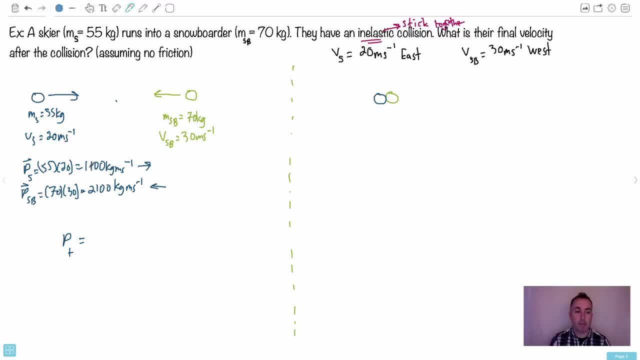 one that's going to win is a snowboarder. so 2100 minus 1100, that's going to give me a thousand. so what i'm going to do then with that number thousand? i have to keep in mind which direction it is. so that gives me a direction to the left, and this is the only thing that's allowed to cross. 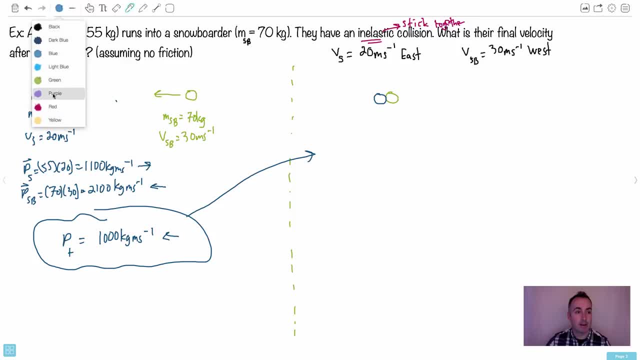 that line, what i mean by that line? that line is going to define before the collision and after the collision. so that way, the only thing that can cross this line, the only thing that's useful, the only thing that's conserved, is this total momentum. so now, 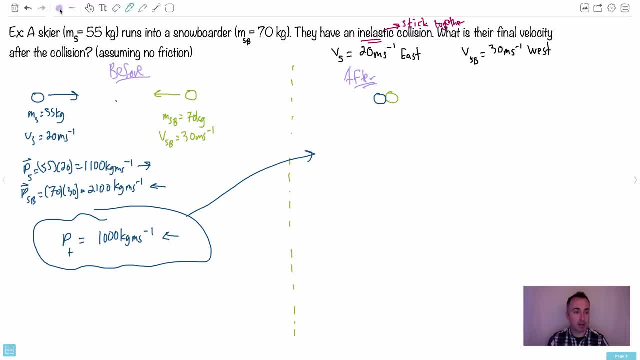 i know that this total momentum is also equal to this same number right here. now. i know that, so maybe i'll write a totally different color now. now i know, then, that p total is equal to 1000 here as well, i even know the direction: it's to the left or west, sorry west. so what happens here? well, they're. 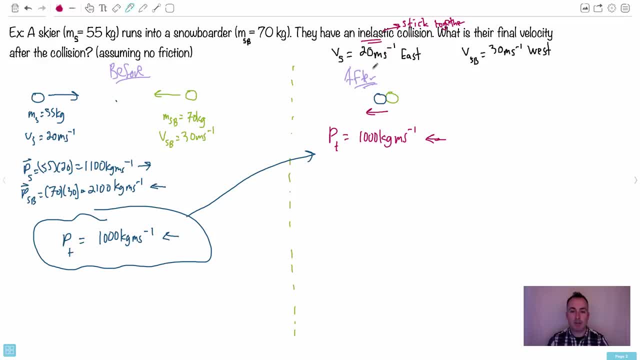 both stuck together. well now, i know they're both going that way and what i can do is figure out. well, i know the momentum equals the mass times, the velocity, but i know that they're together, so it's going to be m1 plus m2, so in other words, it's going to be 55 plus 70, all that times the final velocity, which 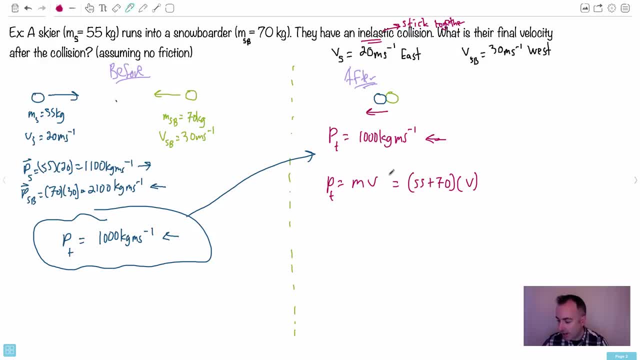 i don't know, remember. i'm actually trying to find that, so i'm going to actually take a look at that and try to do it all here. i can actually put in for pt. here i've got a thousand, so that's going to equal, because that's my total momentum. i know that thousand equals this plus this times v. so 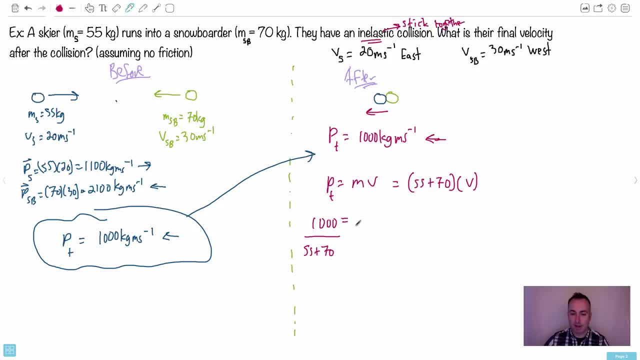 that means that thousand divided by 55 plus 70, uh, that's going to equal v. so i'm going to get out my trusty calculator here and see if i can solve this. so i've got uh 55. what do i have to do? i have to do: a thousand over was 125. 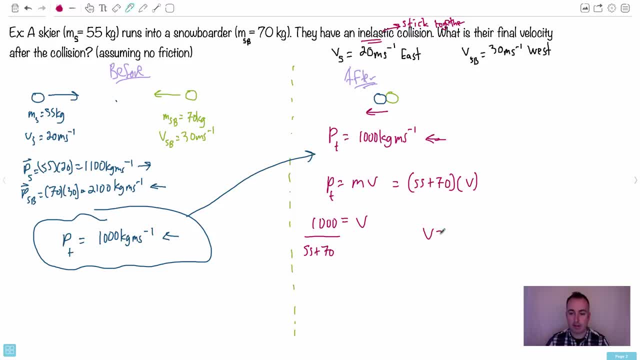 i end up with eight. so my velocity then is eight meters per second, and it's left, so in other words, it's west. that's what's gonna happen. that's gonna be the total velocity, or, sorry, the- of both of them together. So that's how you can use this to solve things. Now comes something. 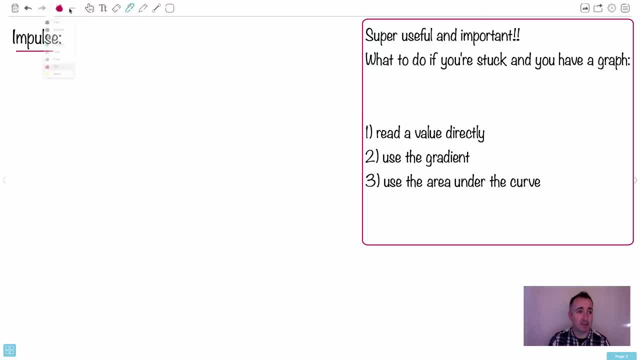 really important, which is impulse. It's something that a lot of students, I think, really struggle with. You have an equation for it. You're actually told impulse. this is in your data booklet: impulse equals. how does it go? It goes f delta t equals. is it m delta v or do? 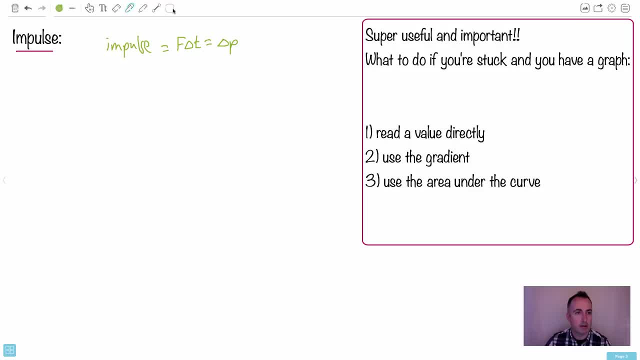 they give you delta p. I think they just say delta p. You have to know that This is the impulse equation. You get this in your data booklet. It looks just like this. So what does this mean? Well, impulse, then, is a change in momentum. That's the key thing. So impulse is a change in. 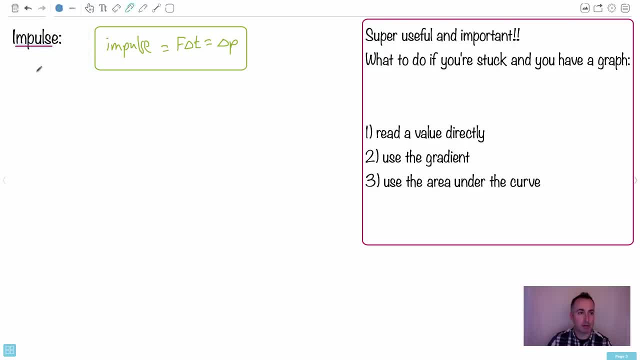 momentum. It's a change in momentum. So if the momentum changes, then there's been an impulse. The important thing is this: force and delta t. So what I'm going to do is I'm going to draw myself a graph of and delta t. An impulse is really like a kick or a push or something like this. So I imagine 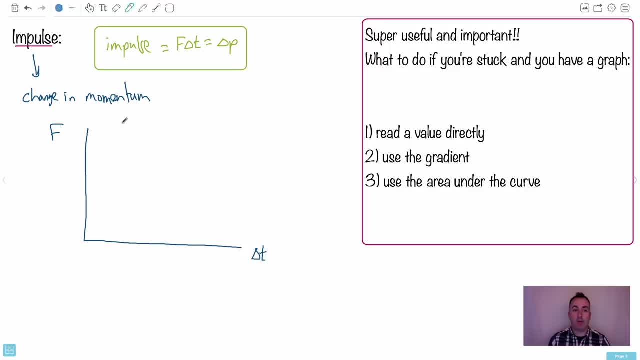 like if I kicked a ball then I would impart a force on that ball in a short amount of time. So therefore you can calculate, then, what the impulse is. So the way the impulse works is, I mean, this graph might be actually a weird shape, It might do some strange shape. 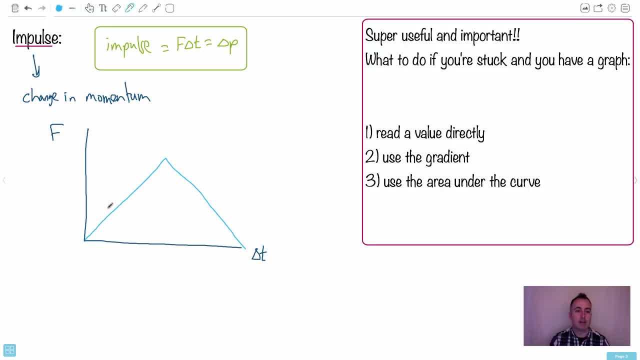 like I don't know what's a common one that they like to use in IB Like that, Like a nice sort of shape like this. And the question is like how do I find the impulse from just this one graph? And that brings up what I think is maybe one of the most useful things. 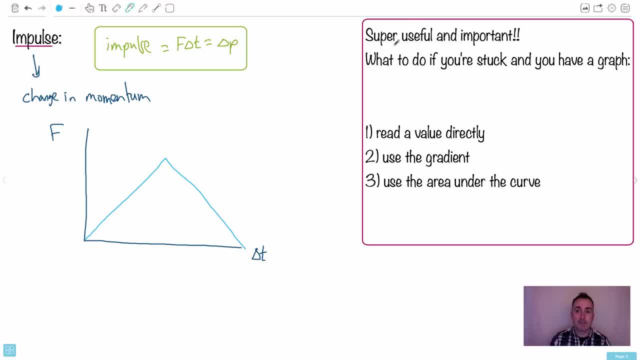 I'm going to show you, maybe in this whole course, is what to do if you're stuck and you have a graph. So this is an example here. This shows up all over the place. I use this trick pretty much everywhere. Whenever I'm not sure what to do, I just do this and it. 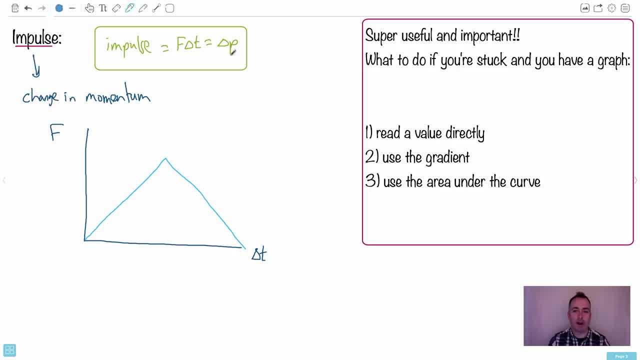 almost always saves the day. So here's what you do When you're stuck and you have a graph. so let's say, I'm looking at a graph, I don't know what this is. okay, It doesn't even matter. I don't know what this is. I don't know what this is. I don't know what. 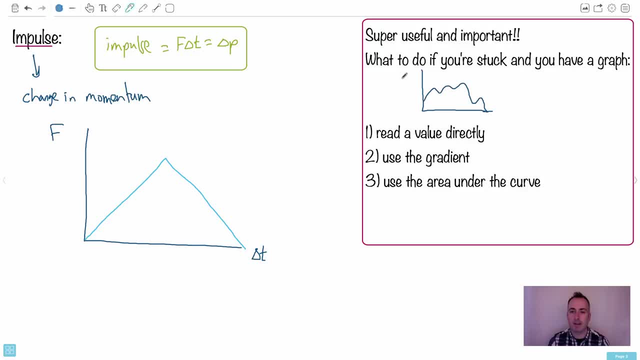 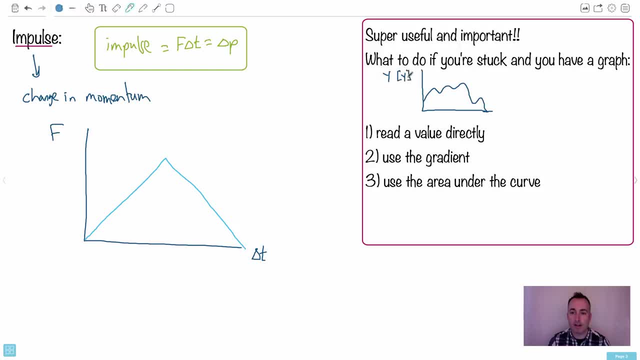 thing called y, whatever that is, and it's got units of y. Like I don't know what, whatever units. We have something x and it's got units of x. So this could be like force, in this case Force which has units of newtons, and delta t which has units of seconds, for example. 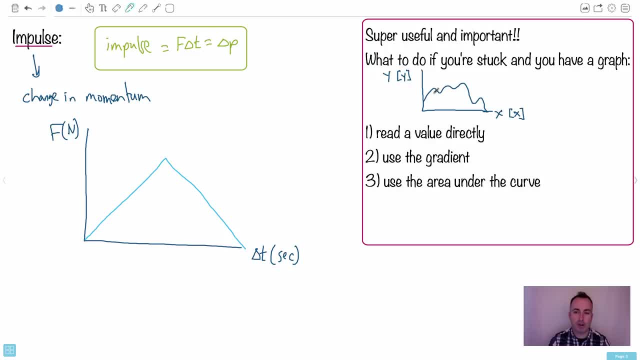 Then you can figure out what to do here. So if you're not sure what to do with a graph, there's only three things you could really do. You could do this, You could do this. You could either read a value directly. So what I mean by that is, let's say, you take 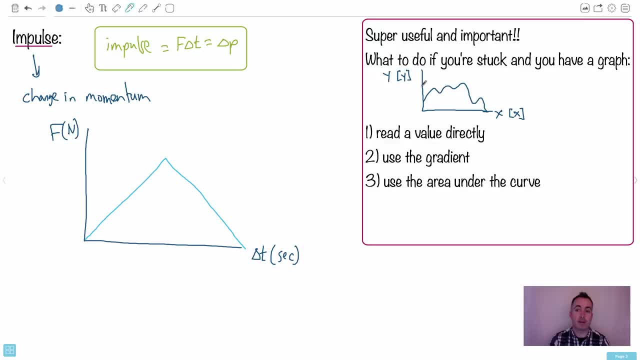 an x thing. you go up here, then you go over there and get the y value, or vice versa. take the y value, read it down, go to the x. You can either read the value directly or you could be using the gradient. If you use the gradient of something, remember that. 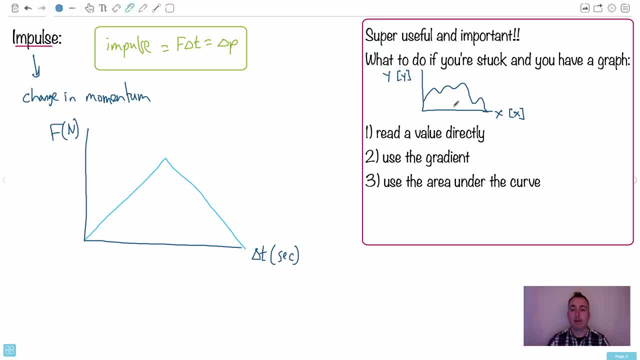 means you have to take a tangent line and then you actually find the gradient of that line. The units of gradient keep this in mind. the units of gradient will have, because remember how gradient goes. Gradient is, isn't it? rise over run. 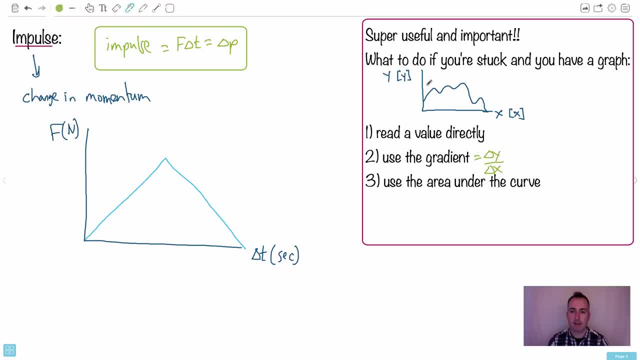 So isn't that equal to delta y over delta x? Like you know, you have to say, take some sort of like. let's say it was this right here. I'll take some sort of gradient right here, And now I'd find out, you know, what was the delta y, what was the delta x? I could 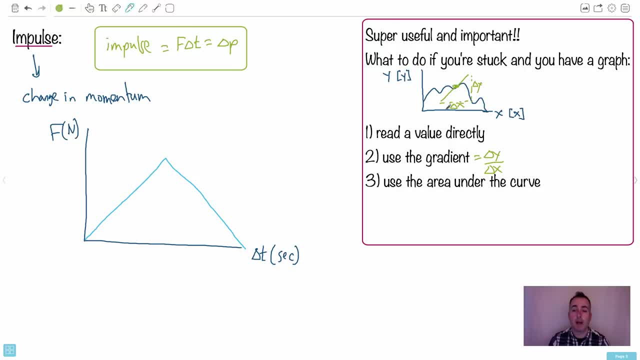 measure that And I could do it right here. if I was wondering something right here, I could take the gradient, but keep in mind what units it'll have. The units it'll have will be units of y divided by units of x, So it'll have those units In this case. if 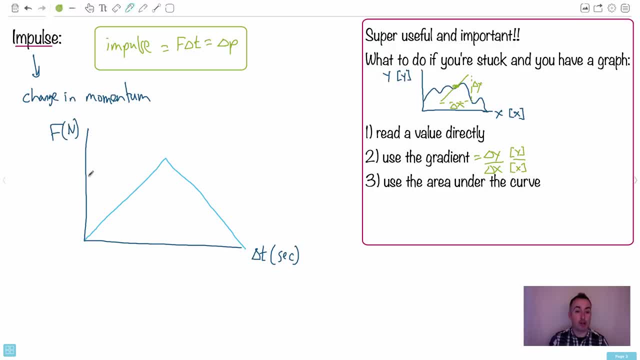 I did the gradient of this bad boy over here, I would have let's see newtons Per second. So in that case it'd be newtons per second. That's one other option. And the last option is you could take the area under the curve. So what I mean by that is 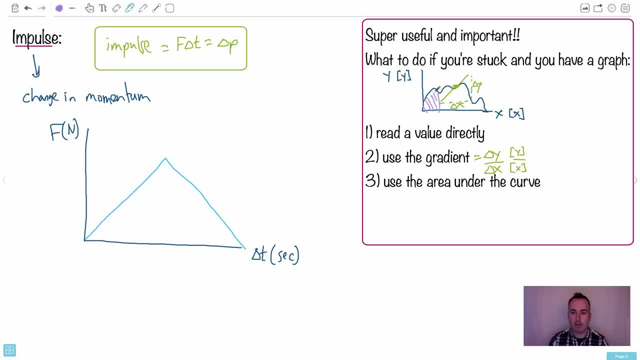 you might actually, I don't know- maybe from here to here, maybe take the area under the curve right here. So the area is going to have units of, because of course you do length times width, right, You do. I should do: area equals x times y, which, in this case, right. 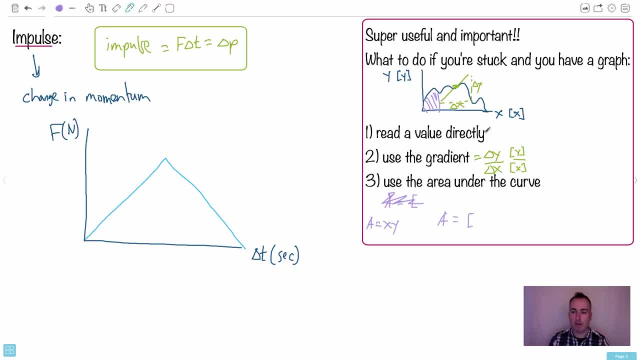 here, then you can say that the area then will have units of whatever x times y. So x was times whatever y was. In other words, these units y times x, It'll have those units. So I basically look at the units to tell me what to do. So if I'm looking for a question, 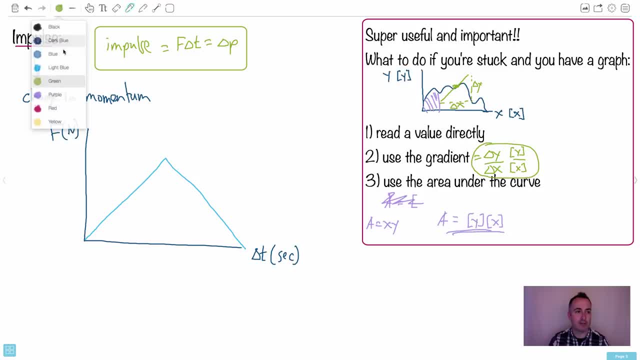 and I'm sort of. they'll often give you a hint on the idea about what kind of things you're looking for. I just take a guess and see: does this get me closer to what I need or farther? So in this case, look at this carefully then. If I've got impulses, f times. 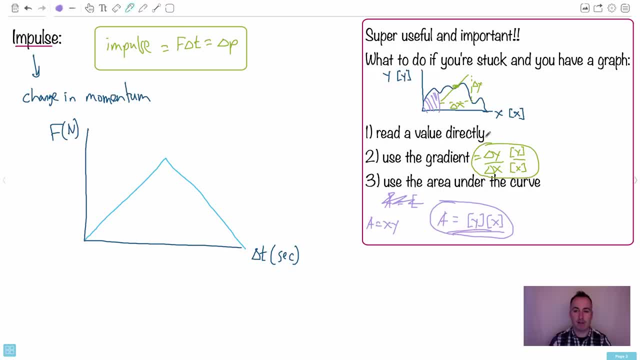 delta t. multiplying. a thing times a thing. is that a reading of value directly gradient or area under the curve- Hope you can see Area under the curve is multiplying, isn't it? So you can then state with this that